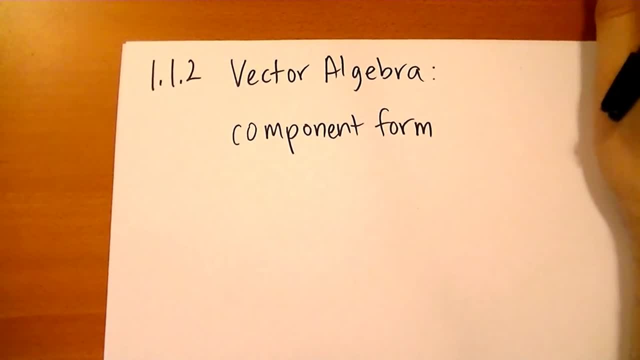 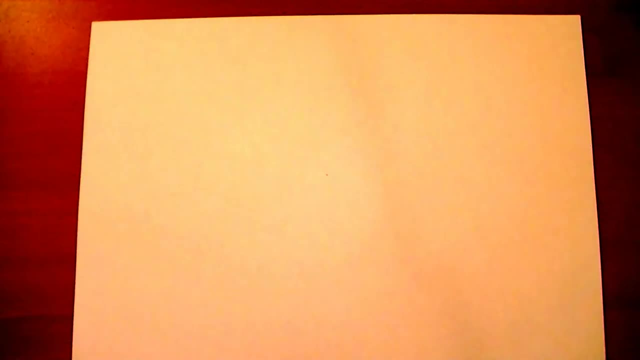 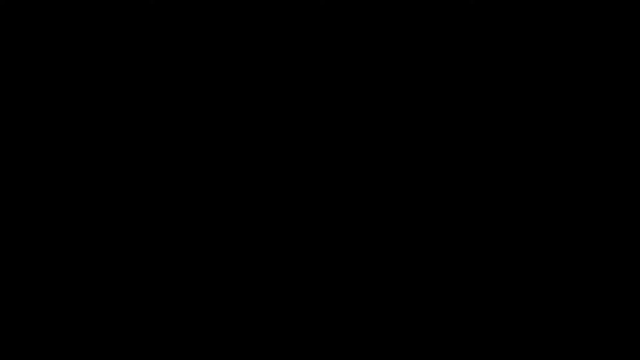 Section 1.12: Vector Algebra in Component Form. So we discussed earlier how to treat vectors in a geometrical sense without using algebra. We talked about what addition, dot products, scalar products, vector products, cross products, what they mean in the geometric world, And now we're going to 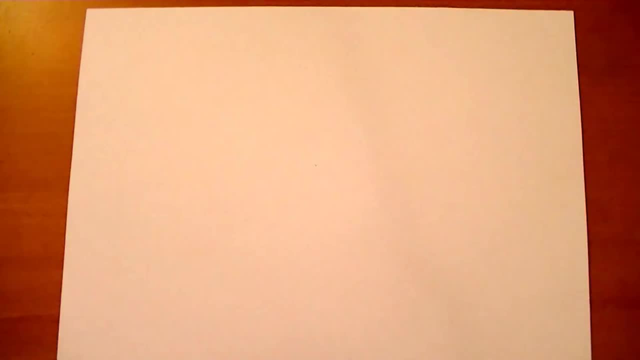 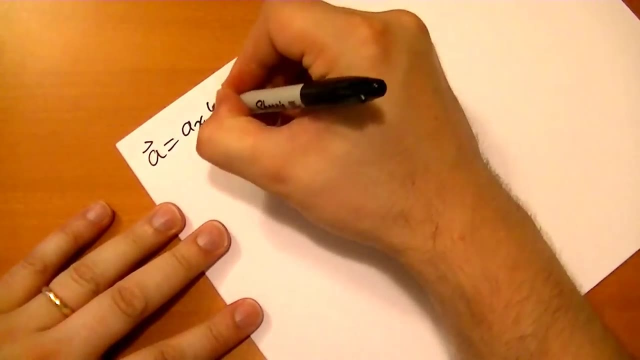 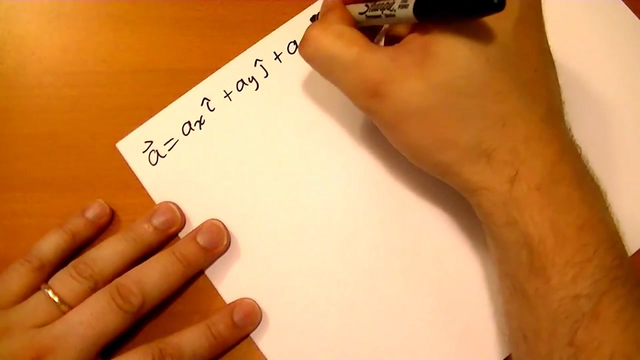 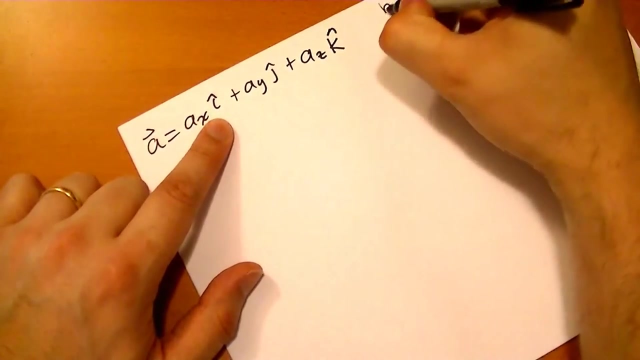 talk about how to write these out in a component form, And what you can do is you can take any vector and you can write it out. A vector is equal to AX times I hat plus AY times, J hat plus AZ times K hat, And what this means is that there's three basis vectors. Let's write that down. 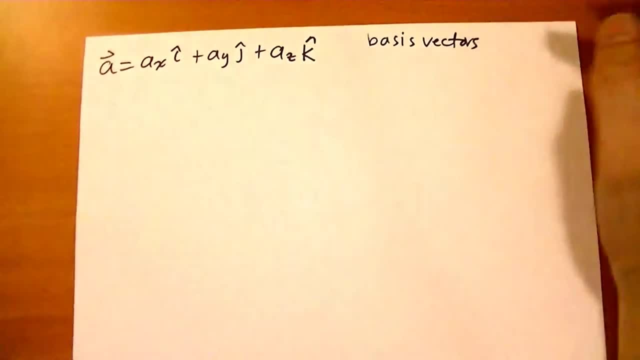 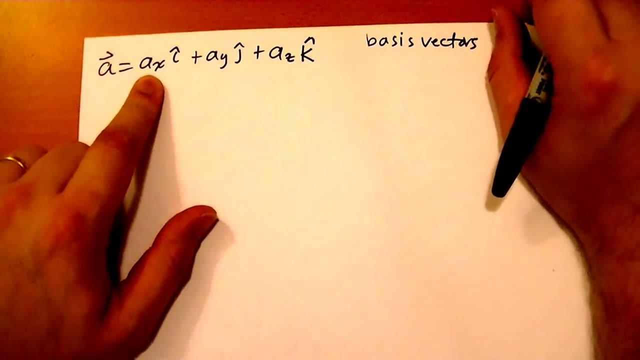 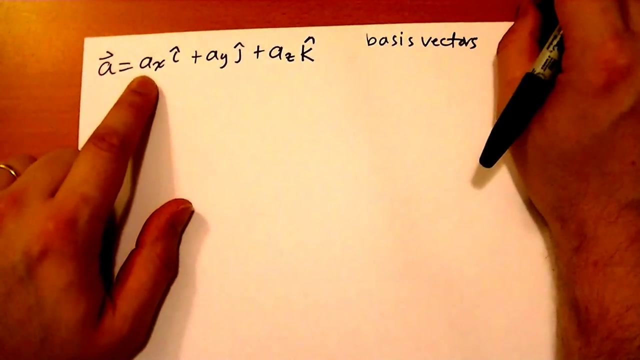 There's three basis vectors. I hat, J hat and K hat. They're each of unit length And A hat A vector can be formed as a sum of scalar products of each of these basis vectors. So AX would be the projection of the A vector on the X axis, AY would be the projection of A on the Y axis and AZ. 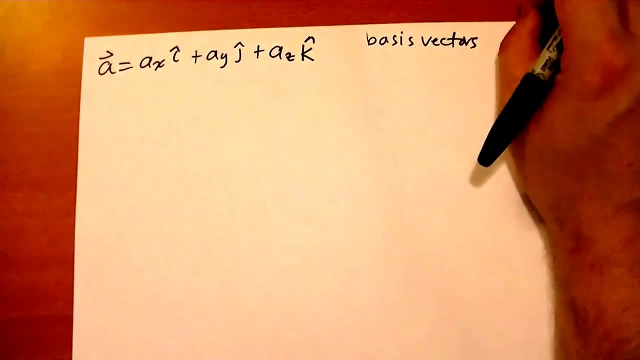 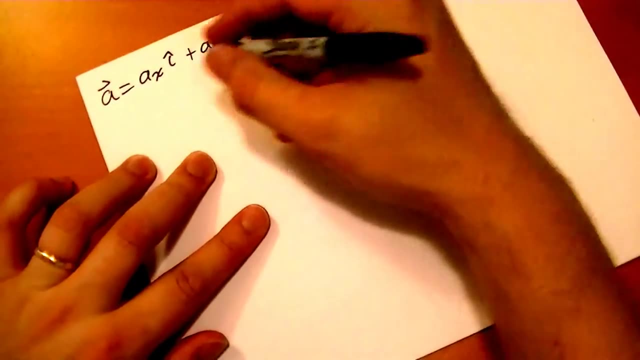 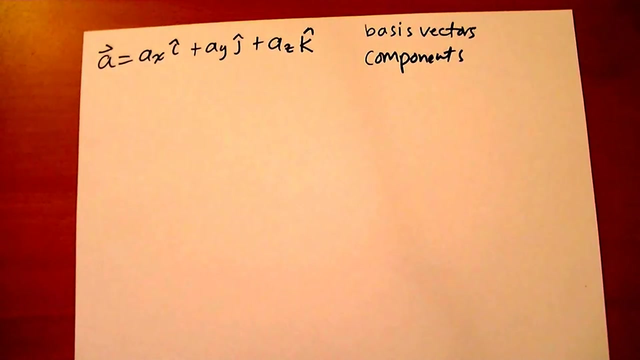 on the Z axis, And if you multiply these by the respective basis vectors, you get your vector in component form. So these are called components In component form. it's a lot easier to work with the math on an algebraic basis rather than. 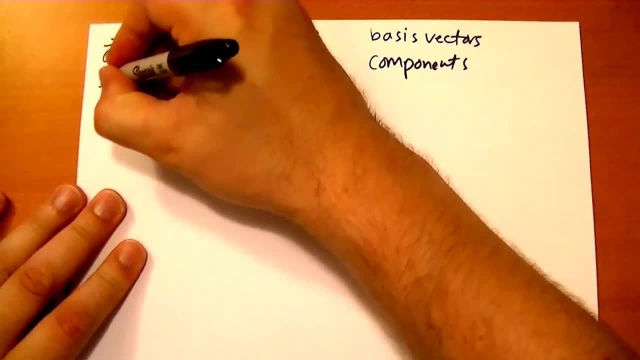 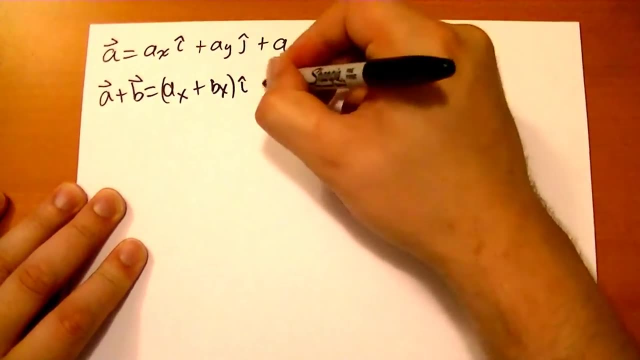 geometrical. So let me give you some examples. So if we want to add two vectors, this is going to be AX plus BX. I hat plus AY plus BY. J hat plus AZ plus BZ, So it's going to be AX plus BX. 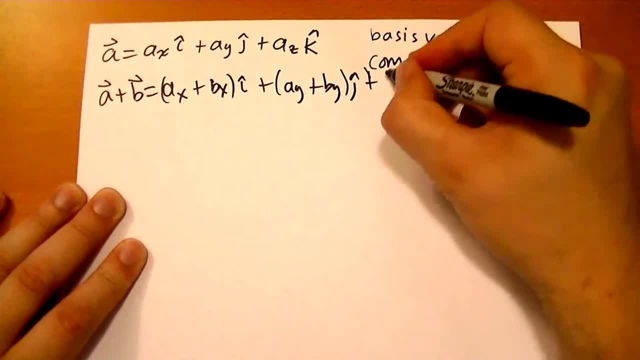 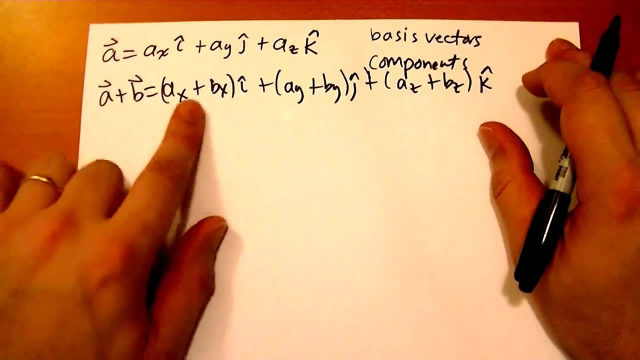 So if we want to add two vectors, this is going to be AX plus BX I hat plus AY plus BY J hat plus AZ plus BZ k hat. and the reason why this works is you just combine like terms, so AXI and BXI are terms from each of these. 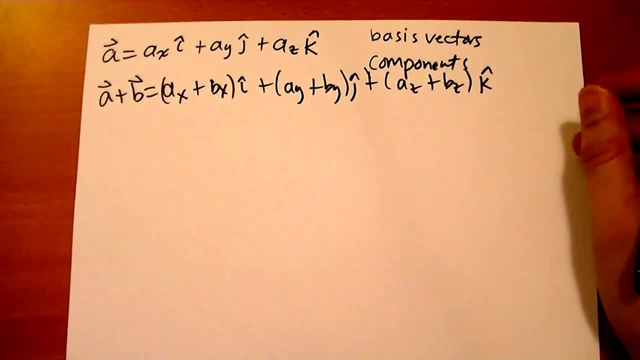 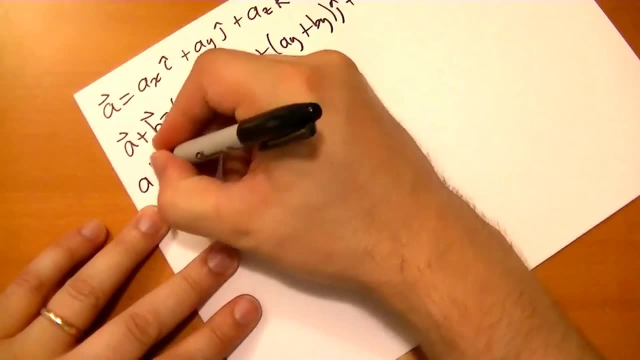 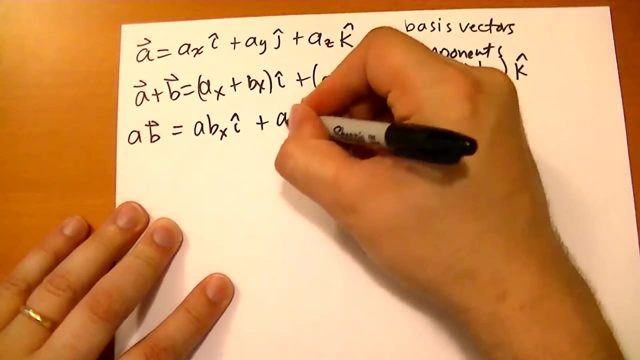 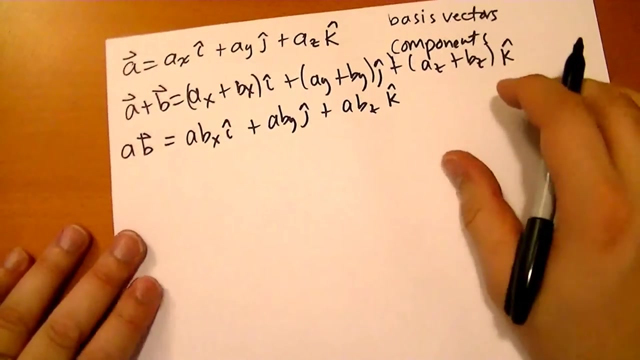 and you just combine like terms and factor out the basis vector. scalar products are simply: you take the scalar times the vector and, as you might expect, you just distribute the scalar. so you get ABXI hat plus ABYJ hat plus ABZK hat. dot products rely on the fact that the basis vectors 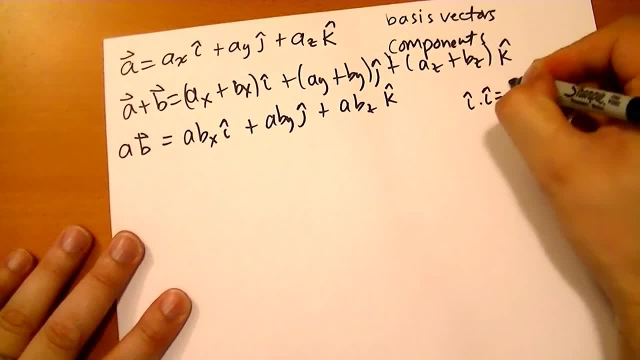 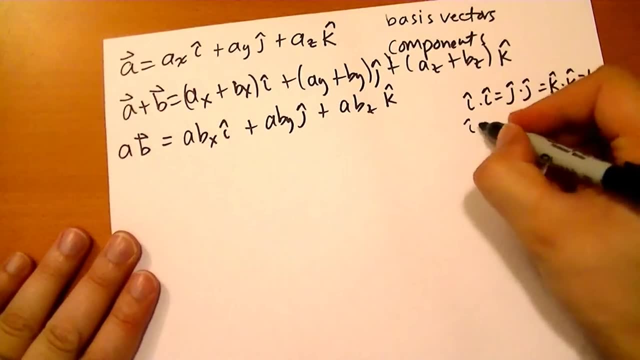 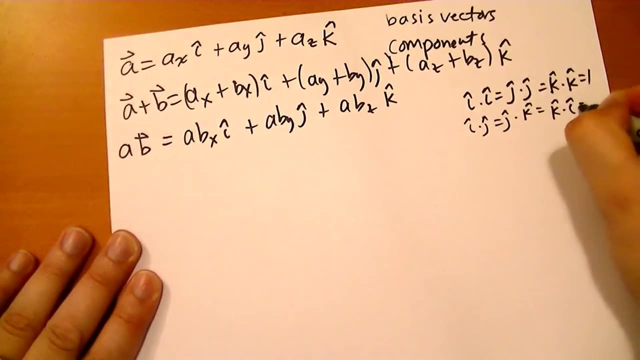 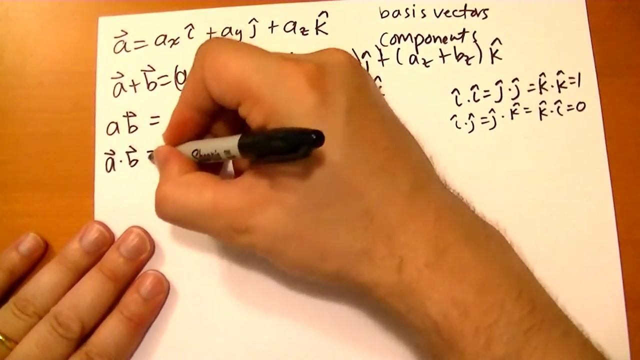 when they dotted with themselves are equal to 1, but when they dot with another basis vector, because they're perpendicular to each other, they're 0. so when you distribute the scalar factors, you get ABXI hat plus ABZK hat. so when you distribute the terms in the dot product, 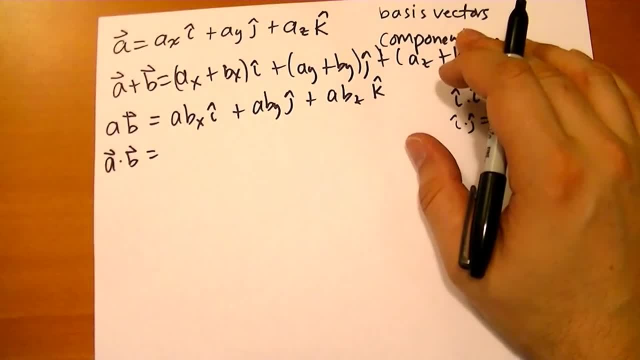 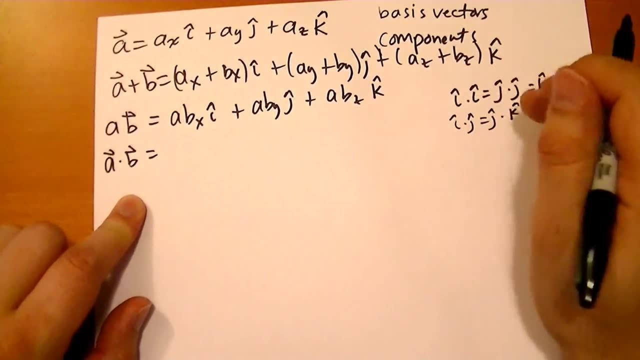 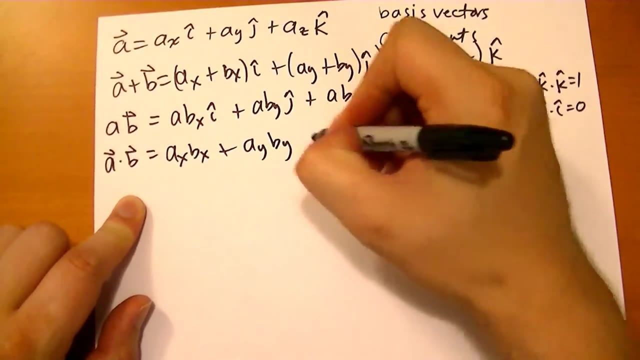 you have nine terms. there's three terms in each one: two, three, four, five, six, seven, eight. there's nine terms, but the only terms that survive are the terms that share the same basis vector, because otherwise they're zero. so you get AXBX plus AYBY. 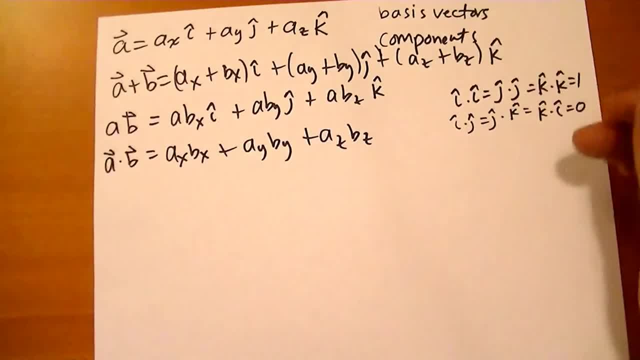 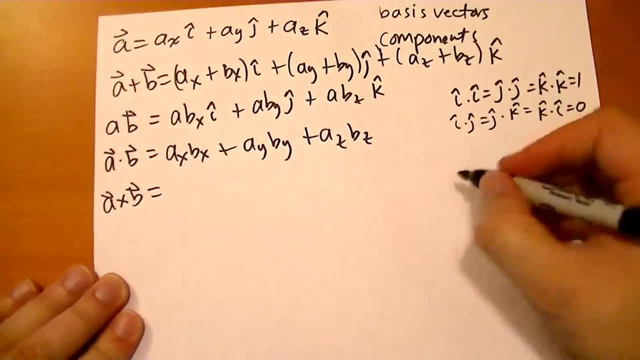 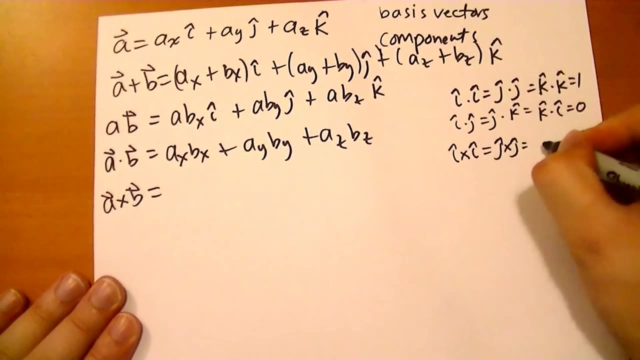 plus AZBZ and, as you expect, that's a scalar, because the dot product is a scalar. the cross product is fairly more involved. it relies on the fact that any basis vector cross itself is going to be zero, because they're parallel with each other, of course. 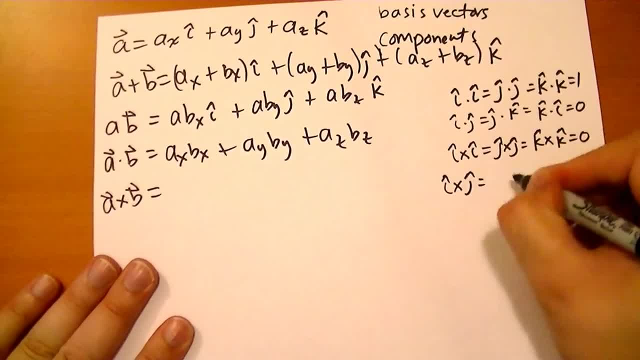 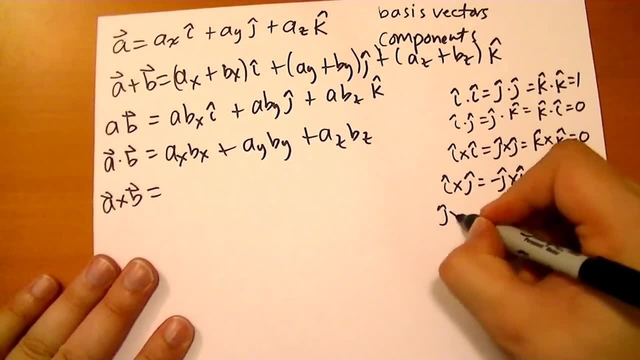 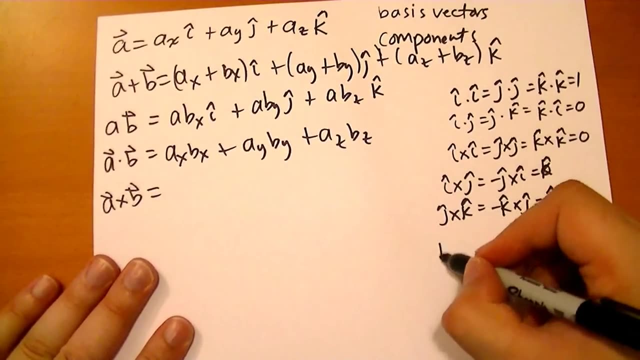 but I hat cross J hat is equal to minus J hat cross I hat. I'm sorry, equals K hat and then J hat cross K hat equals minus K hat cross J hat equals I hat and then K hat cross I hat equals minus I hat cross K hat. 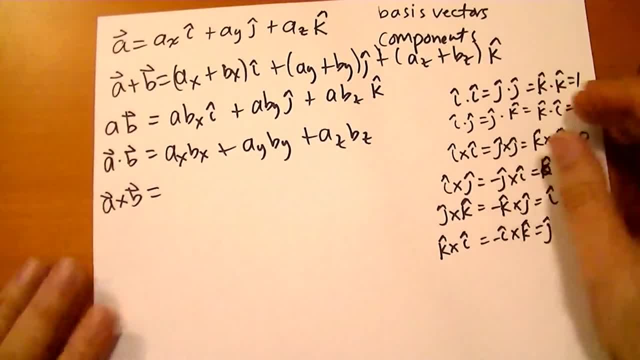 equals J hat. so when you, the terms that survive, the three terms that die, are the terms that are like each other. so when you, when you cross, just it's these opposite of the dot product, the other terms that survive are these: and because it's anti-commutative, 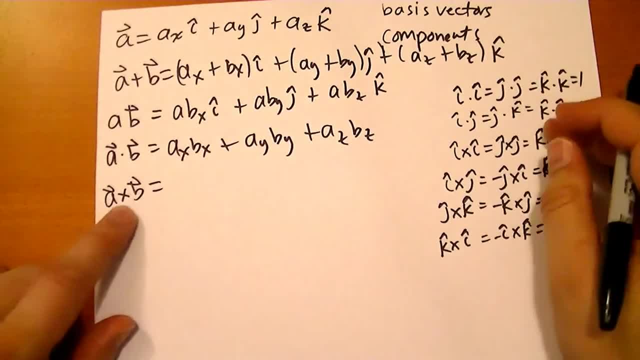 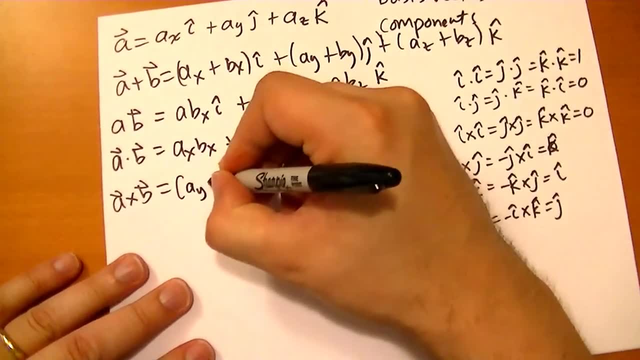 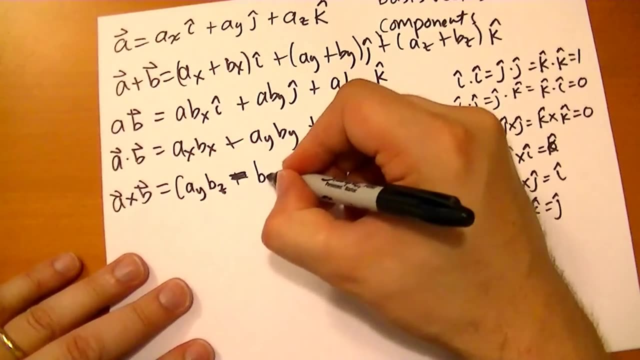 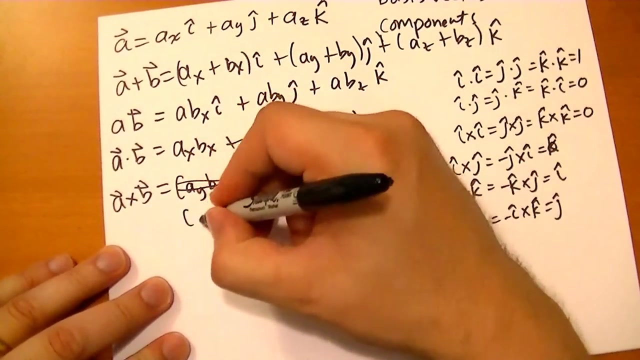 the reverse terms. so AXJ cross BXI is negative, and so you end up with AY BZ. I know I'm going to make a mistake: minus minus, minus, minus B Y. I'm gonna. okay, I always make a mistake when I try to do this from memory. 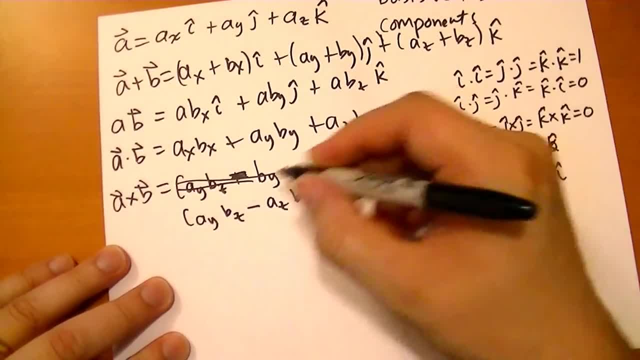 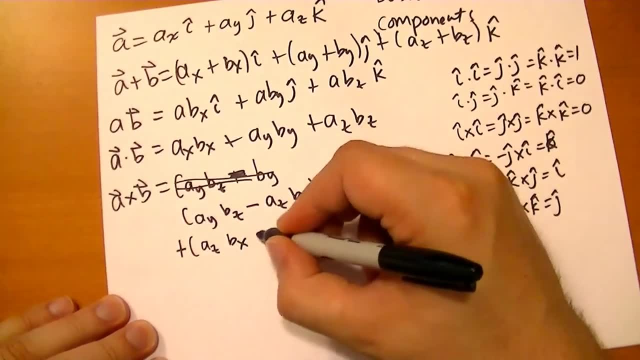 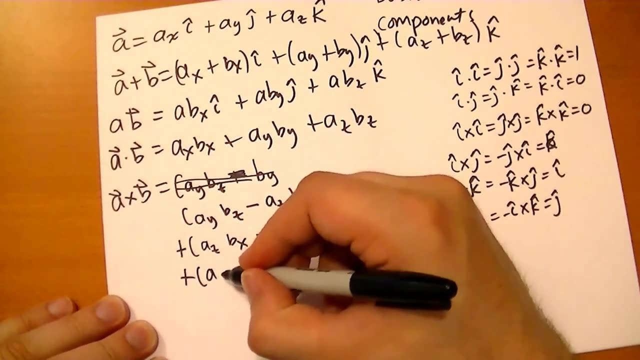 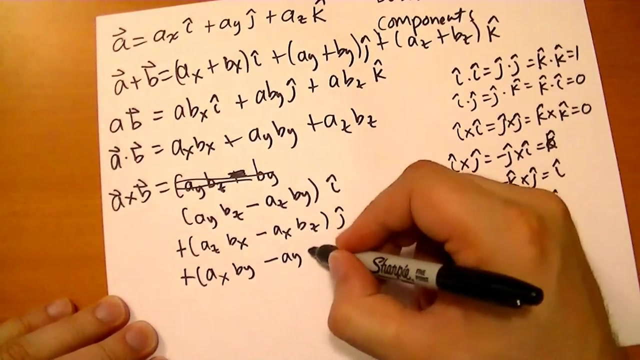 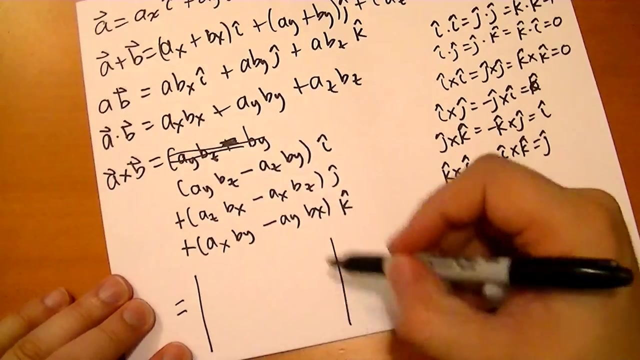 minus AZ BY I hat plus AZ AY bx minus ax bz j-hat. plus ax by minus ay bx k-hat. And this is actually, if you're having a hard time remembering it, you just take the determinant of this, of this matrix. 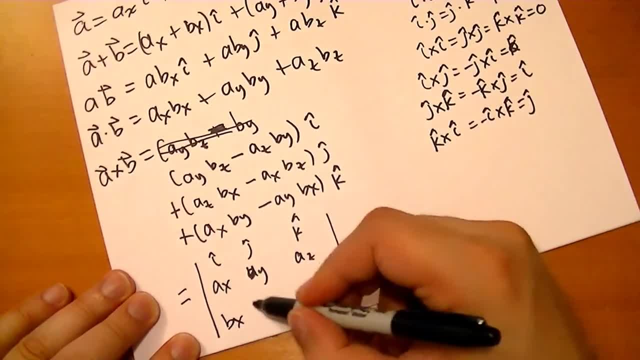 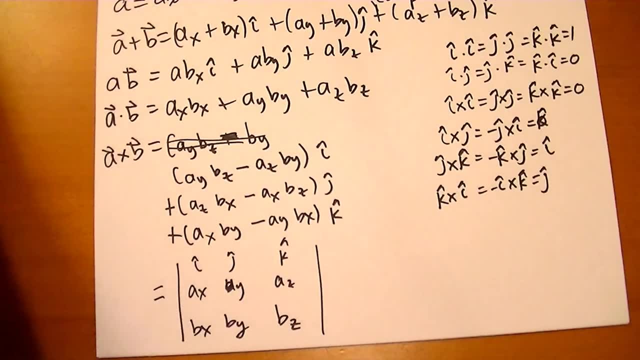 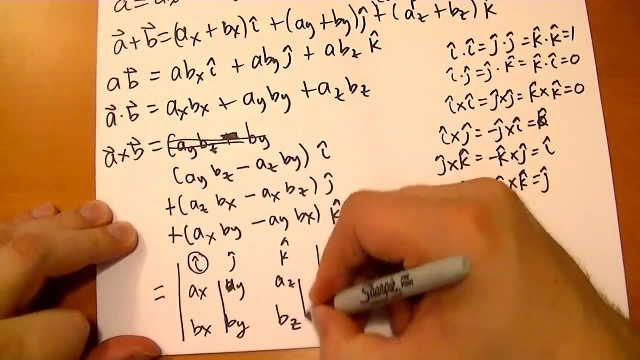 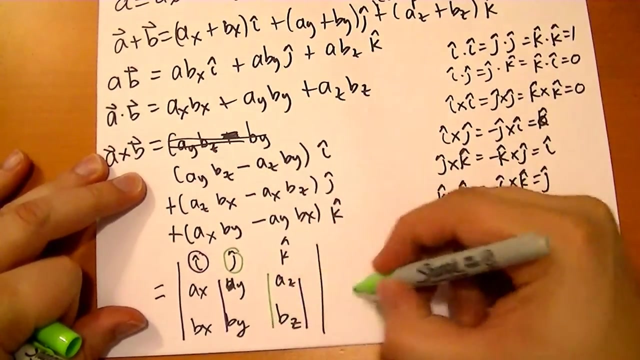 I always do that, And the way you find the determinant is you for three matrix, you first take this one and then you find the determinant of this, and then for the next one, you take this one and multiply it by the determinant of this and we're going to rotate the terms over. so this is ax and bx. 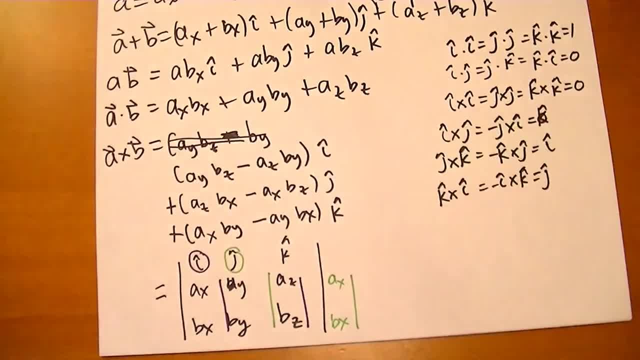 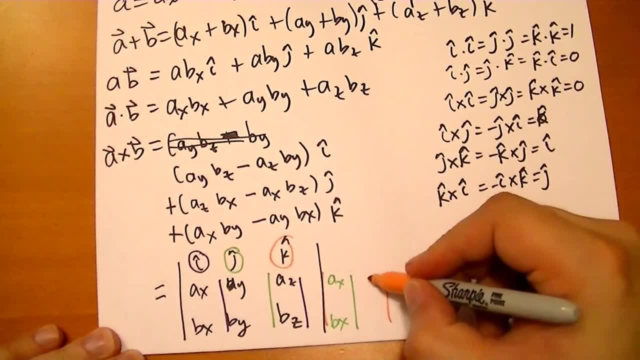 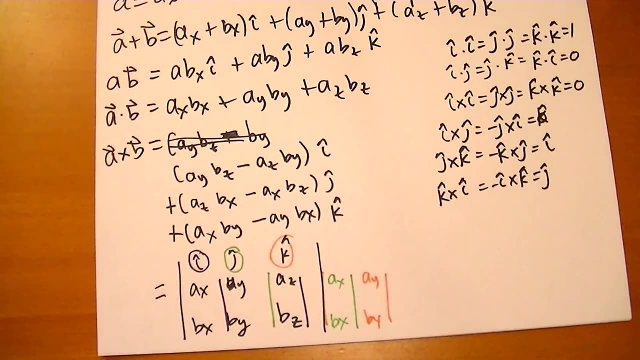 so it's az bx minus ax bz. and for the last term, you start here and take the determinant of this. this is going to be ay and by, so it's ax by minus ay bx. so it's a lot easier to remember the determinant than it is to remember the. 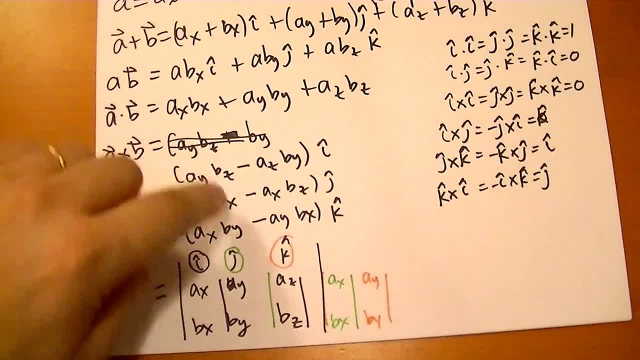 you know I can't even get it right unless I read it. What I actually did is I did the determinant in my head and I got the cross product. So in component form, you're dealing now more with something like algebraic. the derivatives are going to be a lot easier to solve. the integrals are going to be a lot easier to solve. 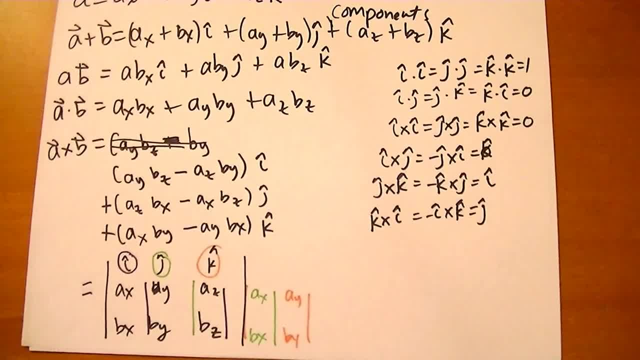 and everything just kind of works out in the end like that. So anyway, hope that helps.